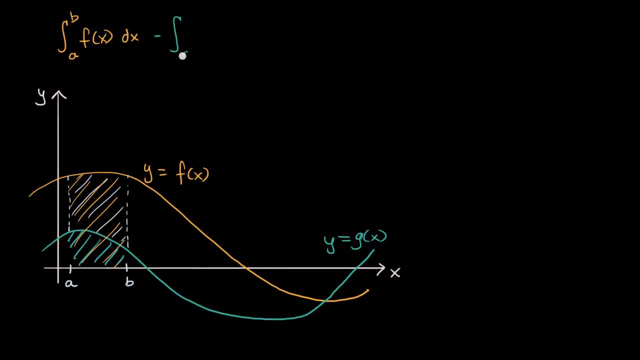 this area right over here, this area right over here, which is equal to, that's the definite integral from a to b, of g, of x, dx. well then, I would net out with the original area that I cared about. I would net out with this area right over here. 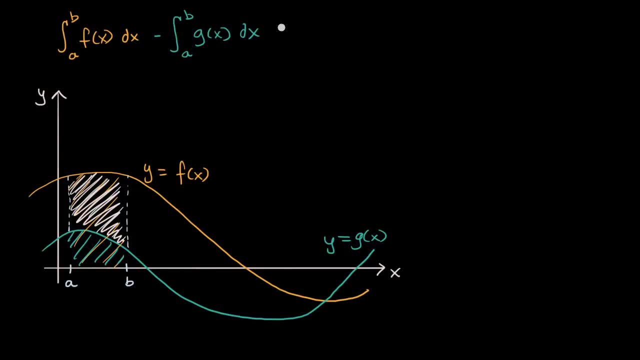 And that indeed would be the case, And we know from our integration properties that we can rewrite this as the integral, from a to b, of- let me put some parentheses here- of f, of x minus g, of x minus g, of x dx. 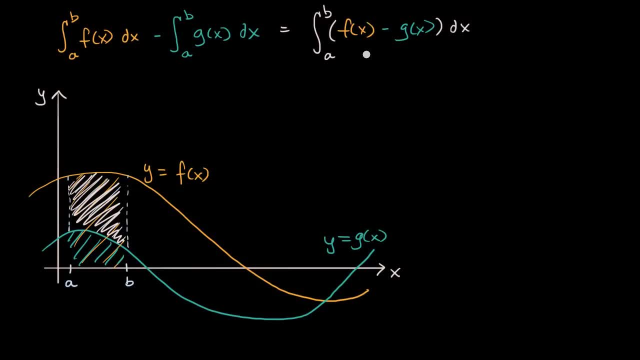 And now I will make a claim to you and we'll build a little bit more intuition for this as we go through this video, But over an interval from a to b where f of x is greater than g of x, like this interval right over here. 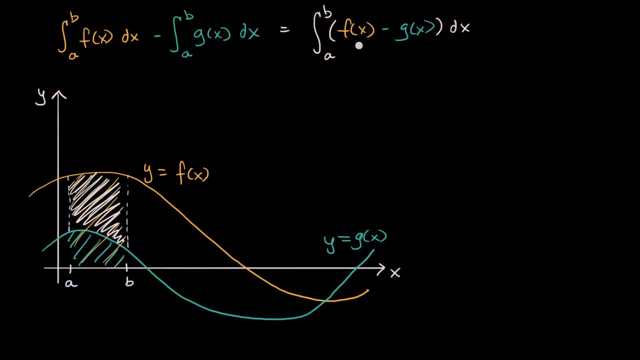 this is always going to be the case, that the area between the curves is going to be the integral for the x interval that we care about, from a to b of f of x minus g of x. So I know what you're thinking You're like okay. 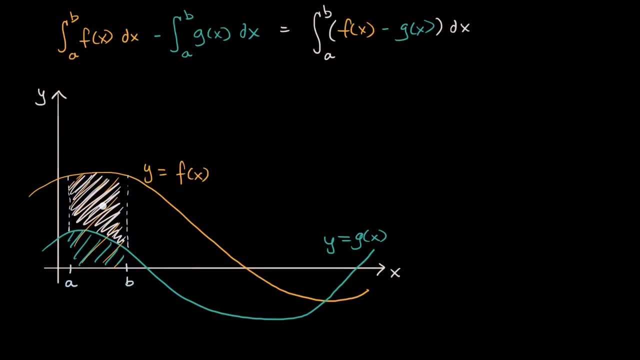 well, that worked when both of them were above the x axis. But what about the case when f of x is above the x axis and g of x is below the x axis? So, for example, let's say that we were to think about this interval right over here. 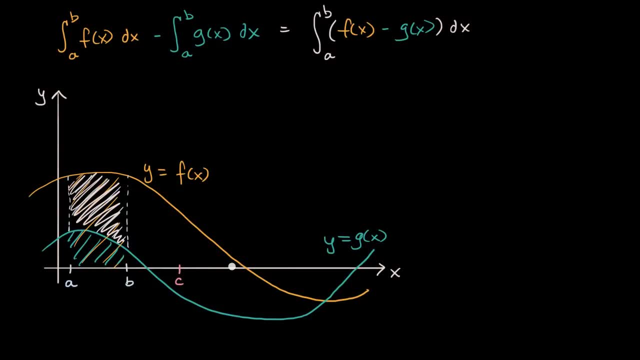 Let's say this is the point C and that's x equals C, This is x equals D, right over here. So what if we wanted to calculate this area that I am shading in right over here? You might say, well, does this actually work? 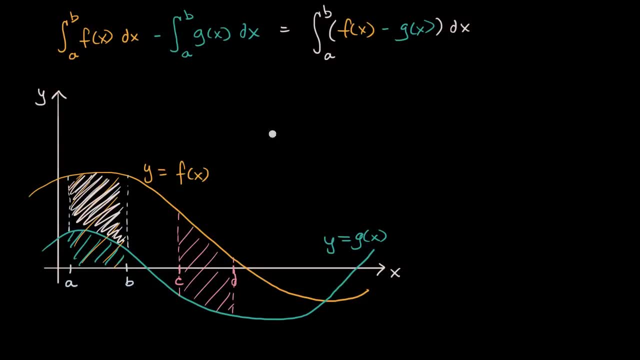 Well, let's think about now what the integral, let's think about what the integral from c to d of f, of x, dx represents. Well, that would represent this area right over here. And what would the integral from c to d of g, of x, dx represent? 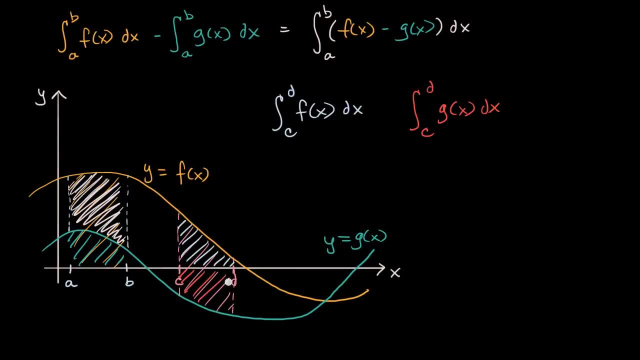 Well, you might say it is this area right over here. but remember, over this interval, g of x is below the x-axis, so this would give you a negative value. But if you wanted this total area, what you could do is take this blue area, which is positive. 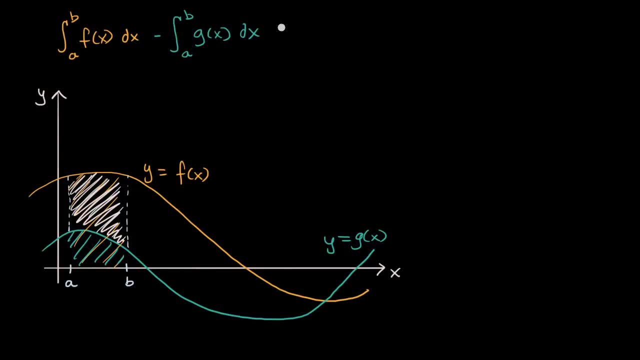 And that indeed would be the case, And we know from our integration properties that we can rewrite this as the integral, from a to b, of- let me put some parentheses here- of f, of x minus g, of x minus g, of x dx. 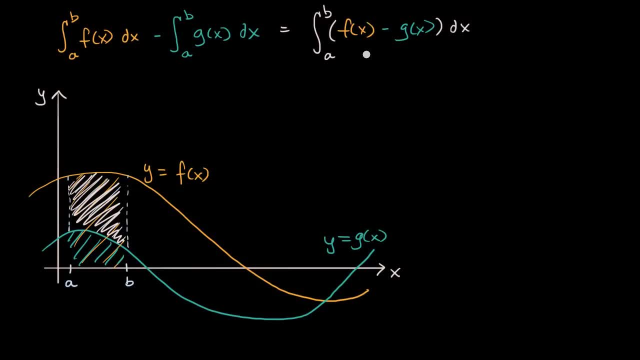 And now I will make a claim to you and we'll build a little bit more intuition for this as we go through this video, But over an interval from a to b where f of x is greater than g of x, like this interval right over here. 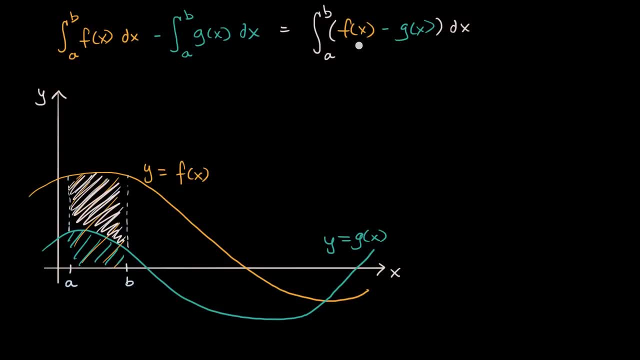 this is always going to be the case, that the area between the curves is going to be the integral for the x interval that we care about, from a to b of f of x minus g of x. So I know what you're thinking. You're like: okay, well, that worked. 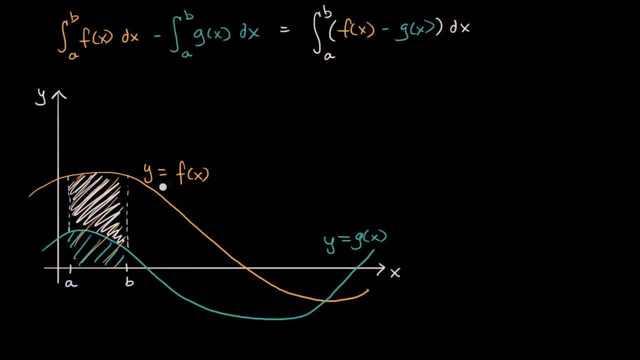 when both of them were above the x axis. but what about the case when f of x is above the x axis and g of x is below the x axis? So, for example, let's say that we were to think about this interval right over here. 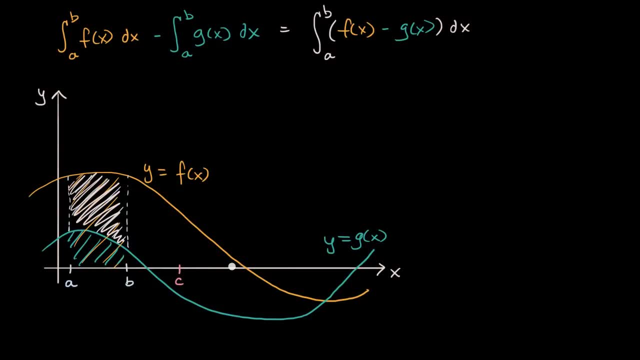 Let's say this is the point c and that's x equals c. This is x equals d, right over here. So what if we wanted to calculate this area that I am shading in right over here? You might say, well, does this actually work? 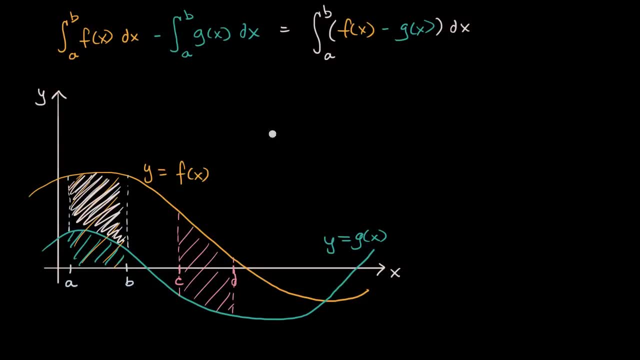 Well, let's think about now what the integral, let's think about what the integral from c to d of f, of x, dx represents. Well, that would represent this area right over here. And what would the integral from c to d of g, of x, dx represent? 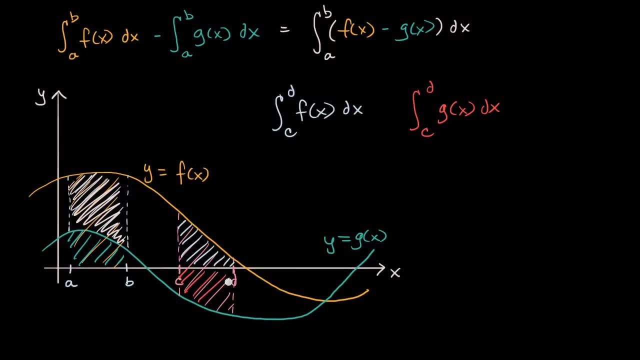 Well, you might say it is this area right over here. but remember, over this interval, g of x is below the x axis, so this would give you a negative value. But if you wanted this total area, what you could do is take this blue area. 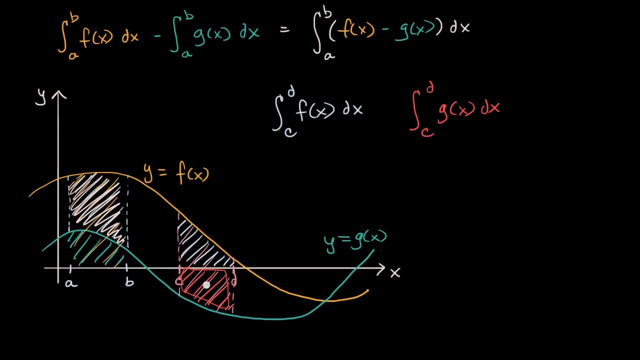 which is positive, and then subtract this negative area, and so then you would get the entire positive area. Well, this just amounted to. this is equivalent to the integral from c to d, dx. So this is the integral from c to d, of f of x minus g of x again. 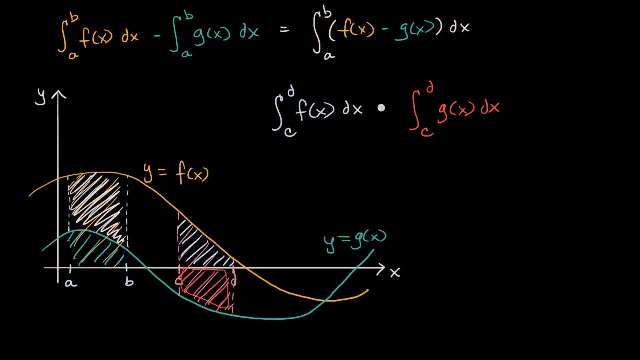 and then subtract this negative area, and so then you would get the entire positive area. Well, this just amounted to. this is equivalent to the integral from c to dx, dx, dx. So this is the integral from c to d, of f, of x, of f of x. 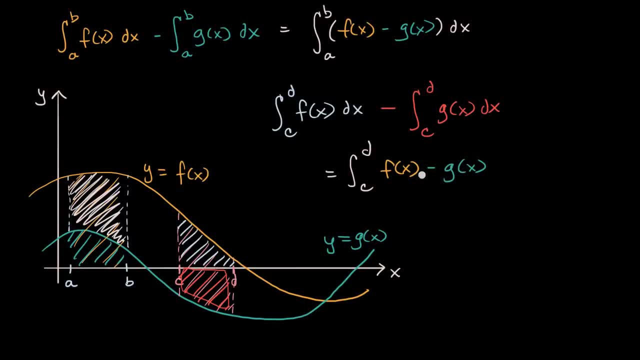 minus g of x, again, minus g of x. Let me make it clear: we've got parentheses there and then we have our dx. So once again, even over this interval when f of x was above the x-axis and g of x was below the x-axis, 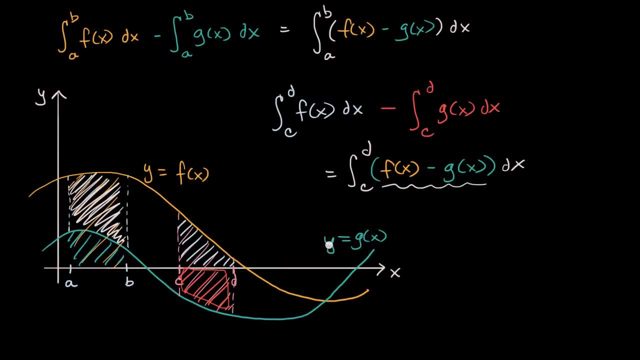 we? it still boiled down to the same thing. Well, let's take another scenario. Let's take the scenario when they're both below the x-axis. Let's take the scenario when they're both below the x-axis. Let's take the scenario when they're both below the x-axis. 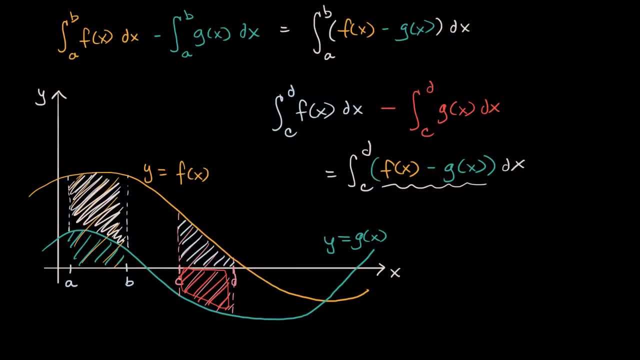 Let's say that we wanted to go from x equals. well, I won't use e, since that is a loaded letter in mathematics, and so is f and g. Well, let's just say: well, I'm kind of running out of letters now. 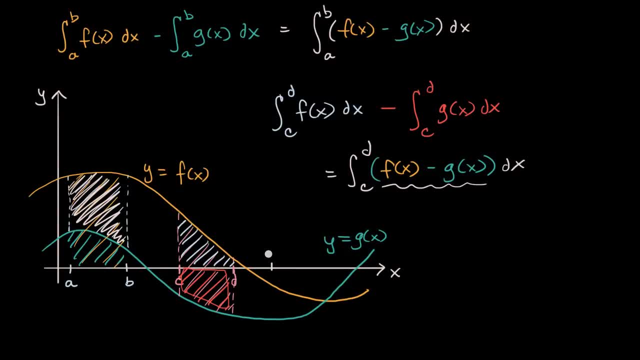 Let's say that I'm gonna go from I don't know. let's just call this m and let's call this n right over here, And we'll n is getting. let's put n right over here. So what I care about. 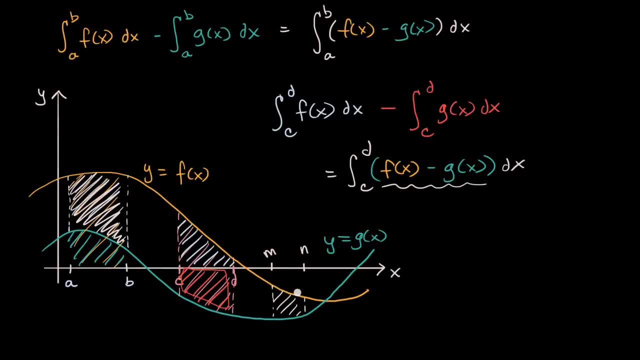 is this area the area once again below f? We're assuming that we're looking at intervals where f is greater than g, so below f and greater than g. Will it still amount to this, with now the endpoints being m and n? 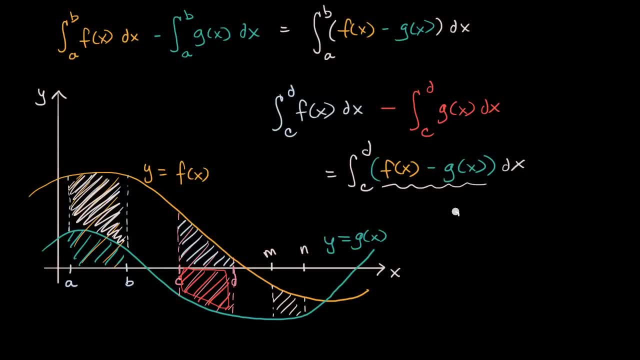 Well, let's think about it a little bit. If we were to evaluate that integral from m to n of- I'll just put my dx here- of f of x minus g of x dx we already know from our integral properties, this is going to be equal to the integral. 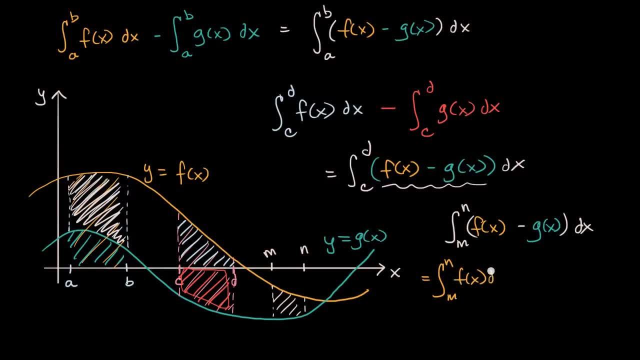 from m to n of f of x dx, minus the integral from m to n of g of x dx. Now let's think about what each of these represent. So this yellow integral right over here, that would give this the negative of this area. 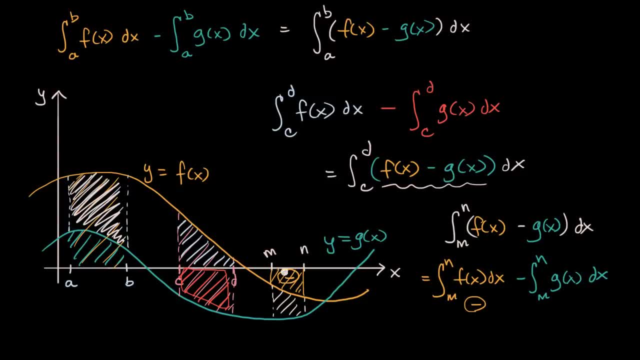 So that would give the negative value here, but the magnitude of it, the absolute value of it would be this area right over there. Now, what would just the integral, not even thinking about the negative sign here, what would the integral of this g of x? 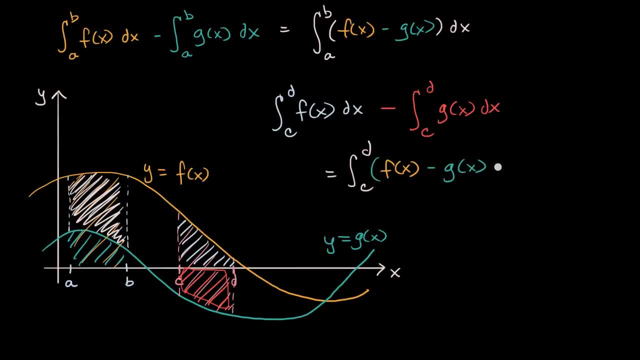 Minus g of x. Let me make it clear: we've got parentheses there and then we have our dx. So once again, even over this interval, when f of x was above the x axis and g of x was below the x axis, 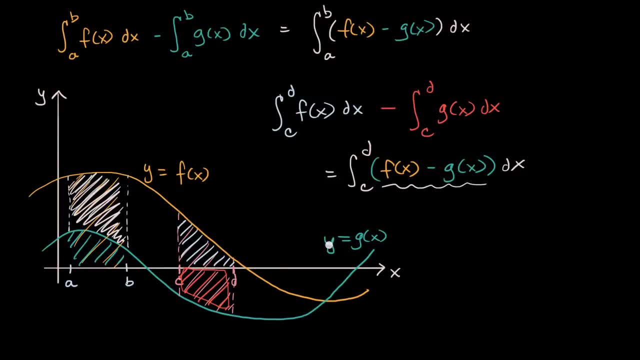 it still boiled down to the same thing. Well, let's take another scenario. Let's take the scenario when they're both below the x axis. Let's say that we wanted to go from x equals. well, I won't use e, since that is a loaded letter. 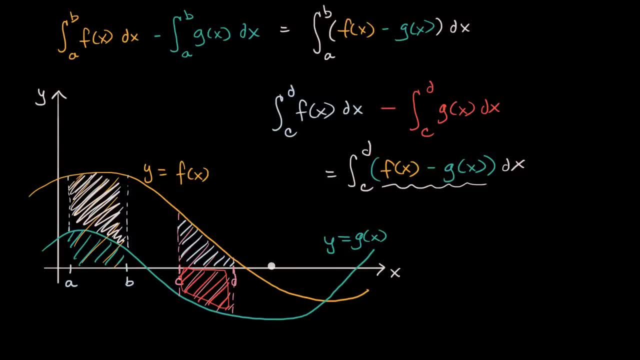 in mathematics, and so is f and g. Well, let's just say: well, I'm kind of running out of letters now. Let's say that I am gonna go from I don't know. let's just call this m and let's call this n, right over here. 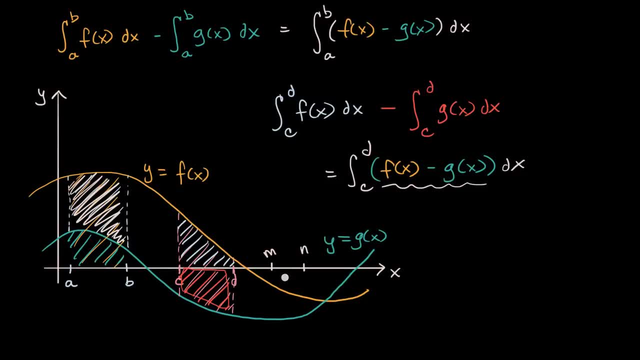 Well, n is getting. let's put n right over here. So what I care about is this area, the area once again below f. We're assuming that we're looking at intervals where f is greater than g, so below f and greater than g. 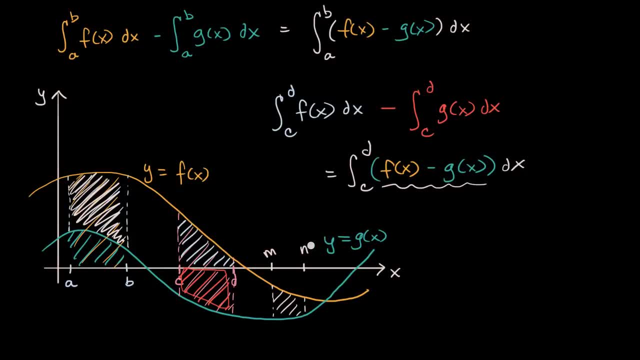 Will it still amount to this, with now the endpoints being m and n? Well, let's think about it a little bit. If we were to evaluate that integral from m to n of- I'll just put my dx here- of f of x minus g of x, 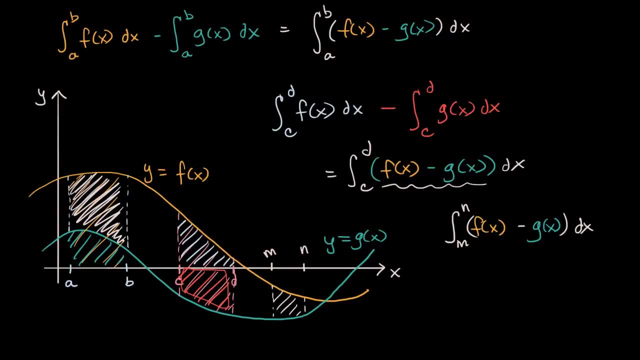 we already know from our integral properties, this is going to be equal to the integral from m to n of f of x dx, minus the integral from m to n of g of x dx. Now let's think about what each of these represent. So this yellow integral right over here, 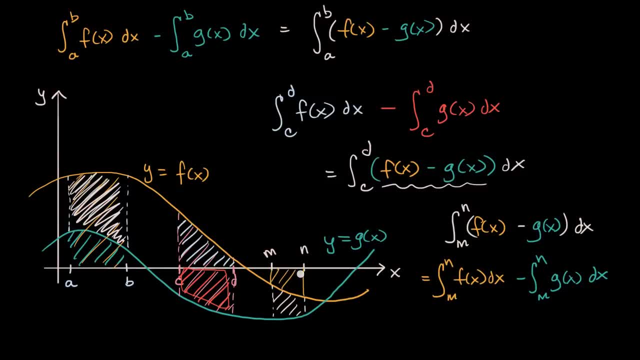 that would give this the negative of this area. So that would give the negative value here, but the magnitude of it, the absolute value of it, would be this area right over there. Now, what would just the integral, not even thinking about the negative sign here.